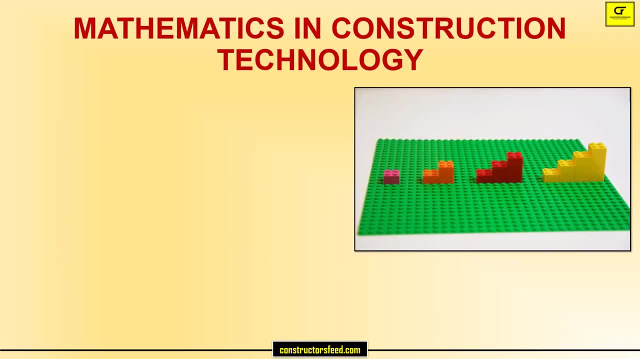 These are the reference books: Mathematics in construction technology. Study of numerical methods for estimating high accuracy in finding the roots and in solving differential equations and their applications. Study of matrix algebra in a best suitable approach for solving large number of equations using transformation methods. 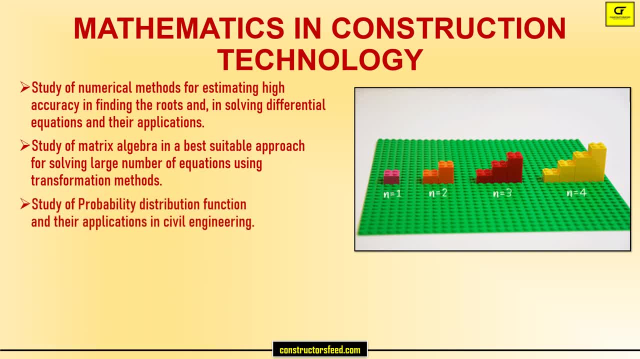 Study of matrix algebra in a best suitable approach for solving large number of equations using transformation methods. Study of array of swimming structures in a class of rectangles. Study of probability distribution function and their applications in civil engineering. Study of concepts of statistical mathematics and their implication in construction engineering. 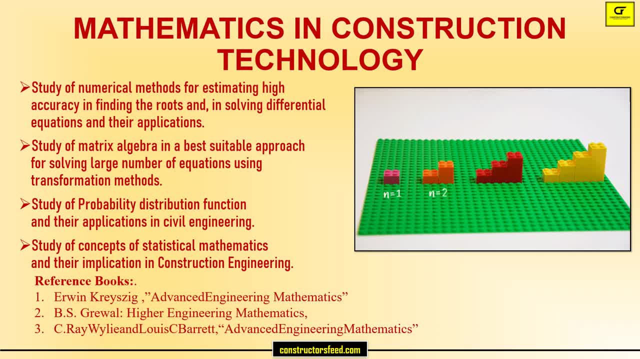 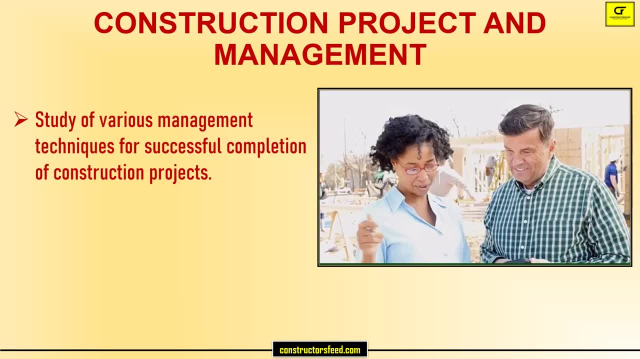 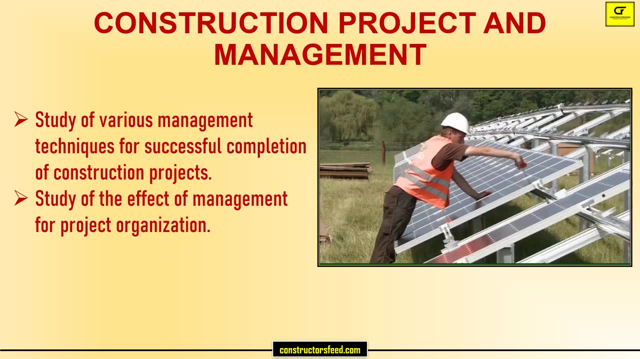 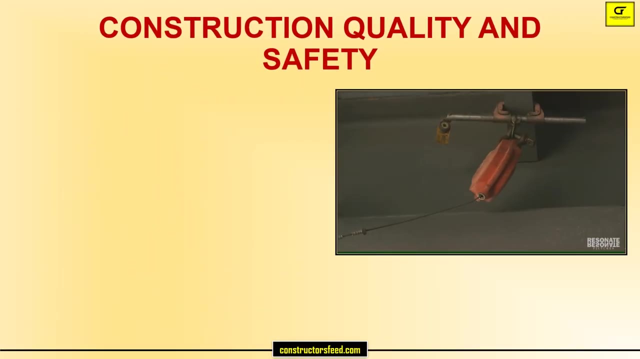 These are the reference books: Construction project and management. Study of various Management techniques for successful completion of construction projects. Study of the effect of management for project organization. These are the reference books. Construction Quality and Safety. Study of Concept of Quality Management and its Implications. 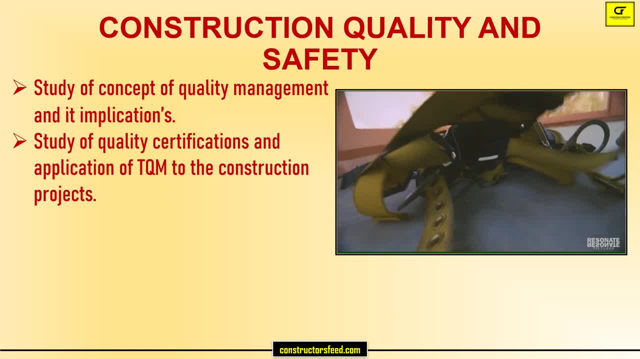 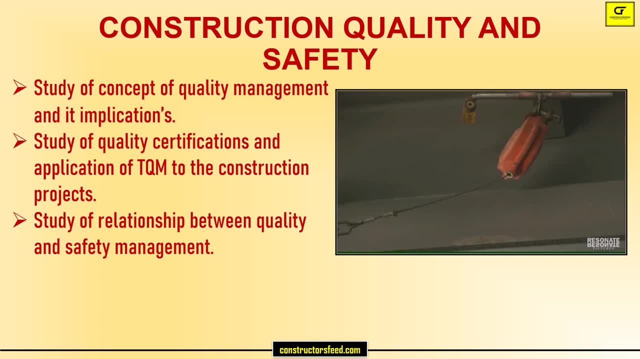 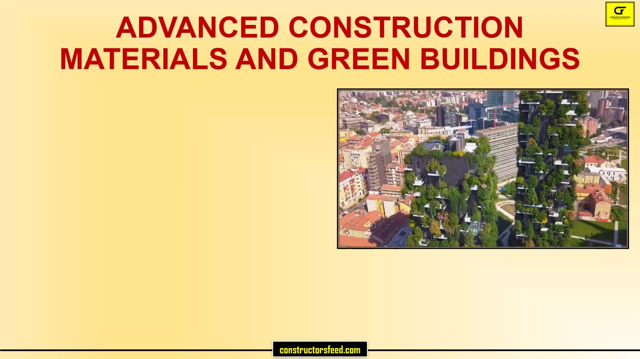 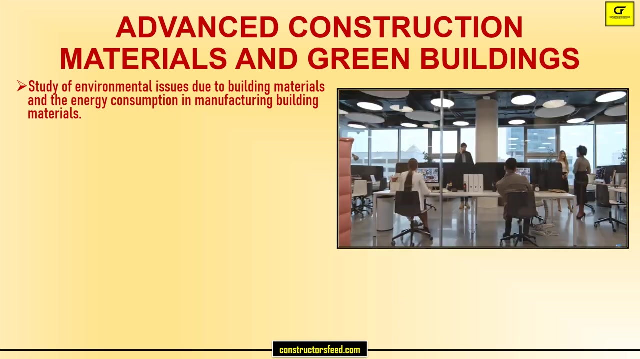 Study of Quality Certifications and Application of TQM to the Construction Projects. Study of Relationship between Quality and Safety Management. These are the reference books: Advanced Construction Materials and Green Buildings. Study of Environmental Issues due to Building Materials and the Energy Consumption in Manufacturing Building Materials. 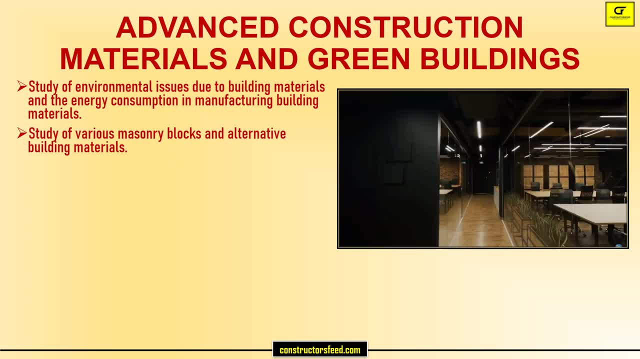 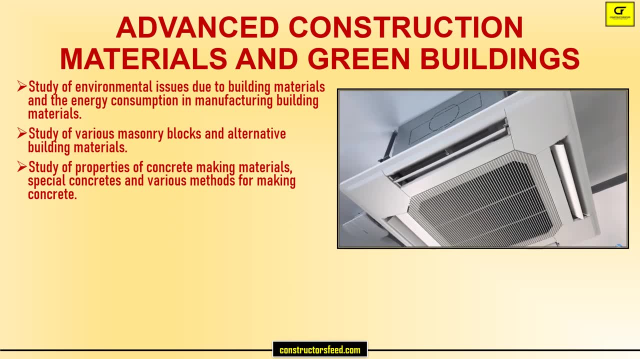 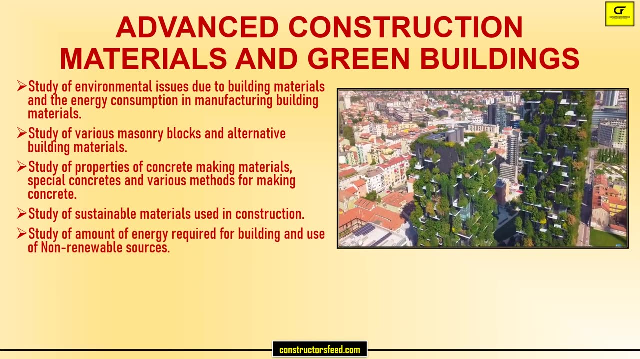 Study of Various Masonry Blocks and Alternative Building Materials. Study of Properties of Concrete Making Materials, Special Concretes and Various Methods for Making Concrete. Study of Sustainable Materials Used in Construction. Study of Amount of Energy Required for Building and Use of Non-Renewable Sources. 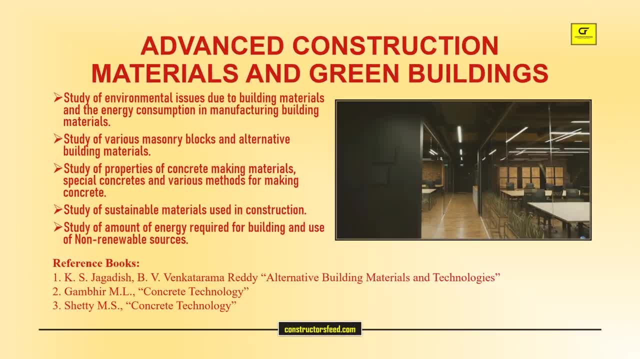 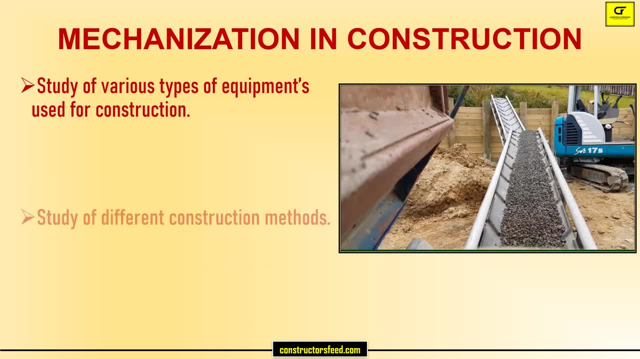 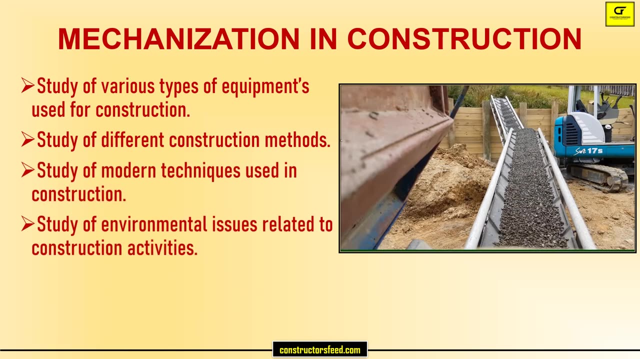 These are the reference books: Mechanization in Construction. Study of Various Types of Equipments Used for Construction. Study of Different Construction Methods. Study of Modern Techniques Used in Construction. Study of Environmental Issues Related to Construction Activities. These are the reference books. 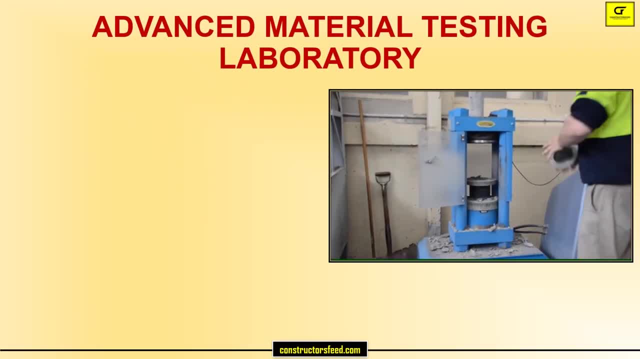 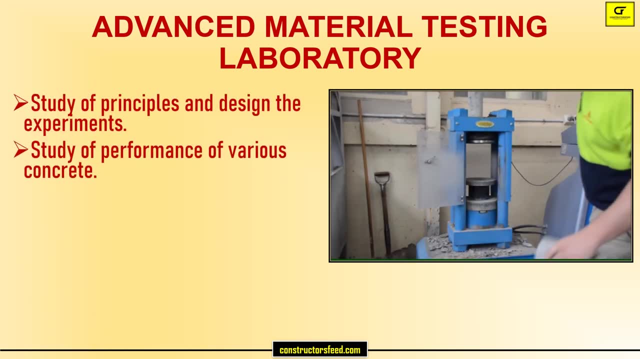 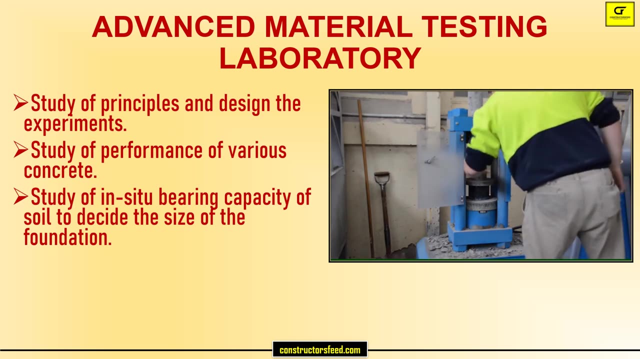 Advanced Materials Testing Laboratory Advanced Material Testing. Laboratory Study of Principles and Design the Experiments. Study of Performance of Various Concrete. Study of In-Situ Bearing Capacity of Soil to Decide the Size of the Foundation. These are the reference books: Construction Economics and Finance. 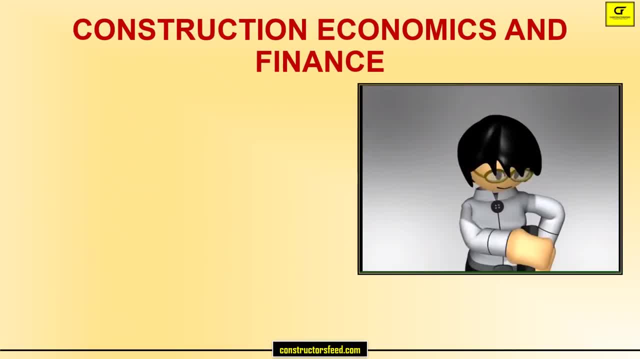 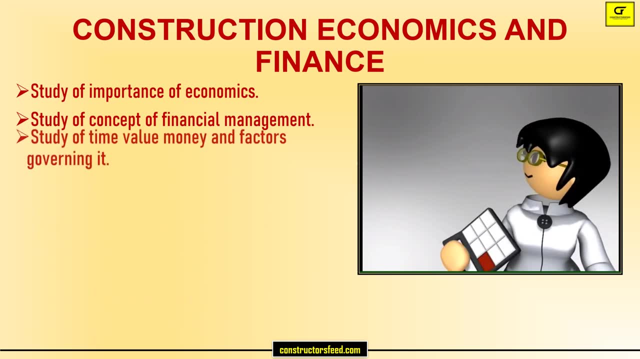 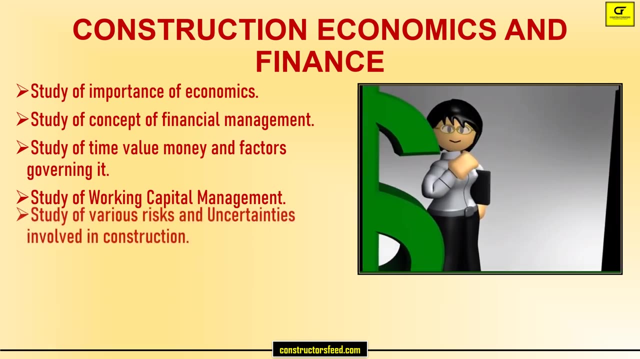 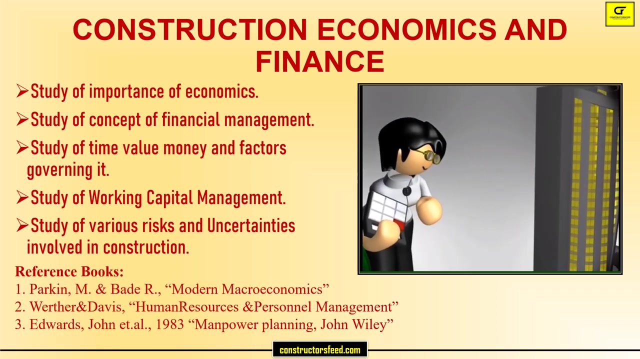 Construction Economics and Finance. Study of Importance of Economics. Study of Concept of Financial and Economic sucker management. study of time, value, money and factors governing it. study of working capital management. study of various risks and uncertainties involved in construction. these are the reference books. pre-engineered construction. 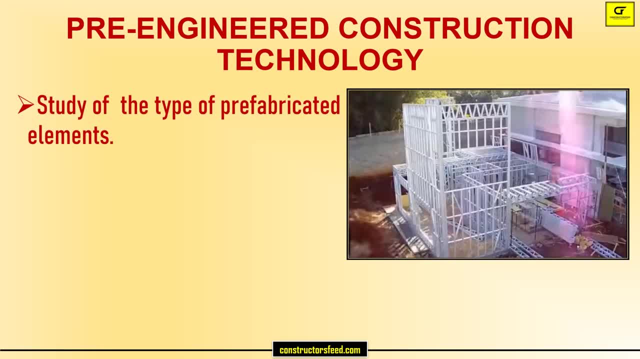 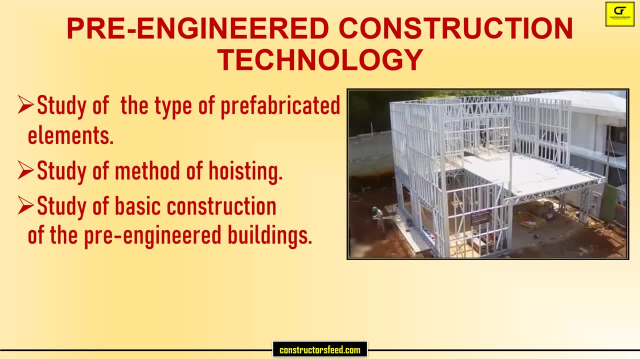 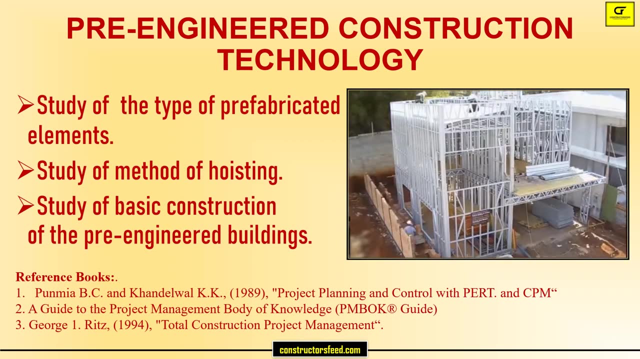 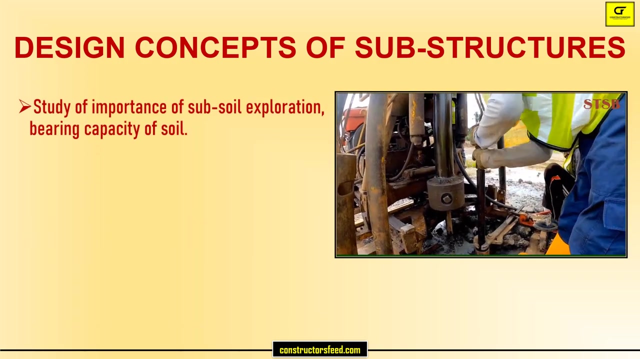 technology. study of the type of prefabricated elements. study of method of hoisting. study of basic construction of the pre-engineered buildings. these are the reference books. design concepts of substructures. study of importance of subsoil exploration, bearing capacity of soil. study of design of shallow foundation and deep 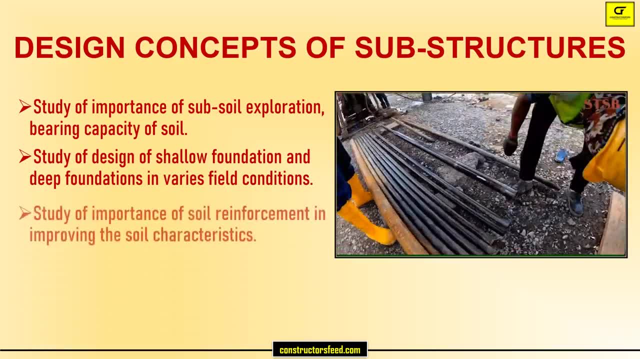 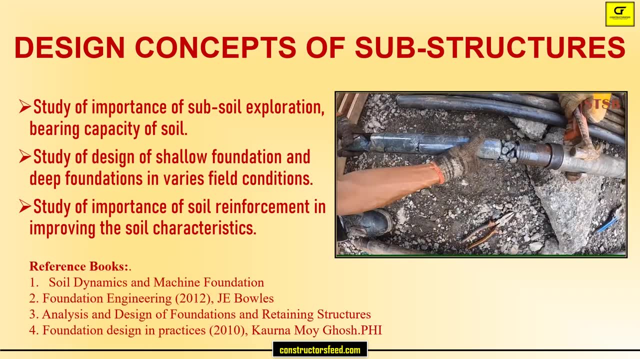 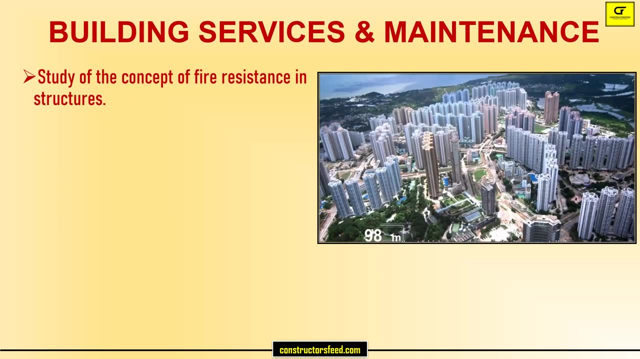 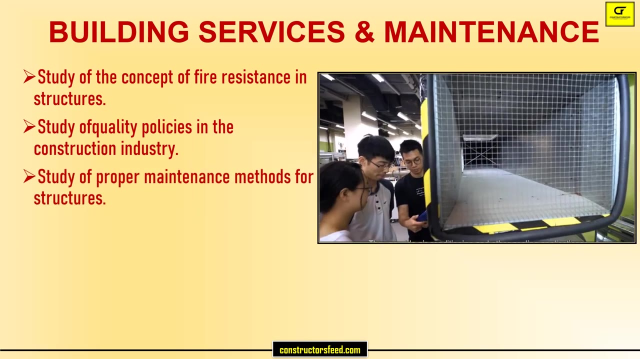 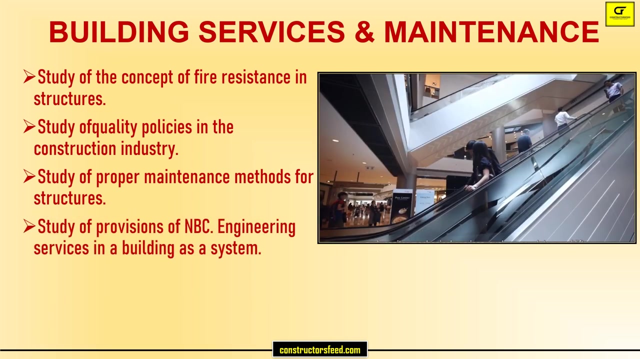 foundations in various field conditions. study of importance of soil reinforcement in improving the soil characteristics. these are the reference books. building services and maintenance. study of the concept of fire resistance in structures. study off quality policies in the construction industry. study of proper maintenance methods for structures. study of provisions of nbc engineering services in a building as a system. 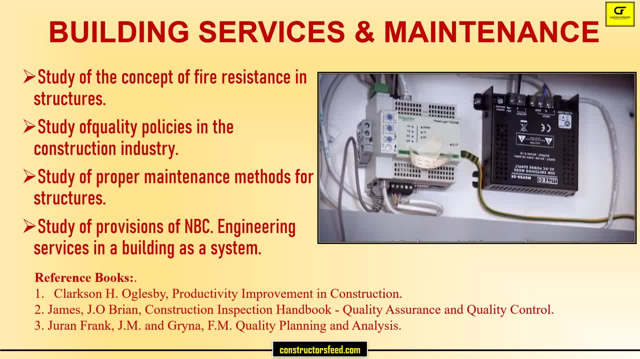 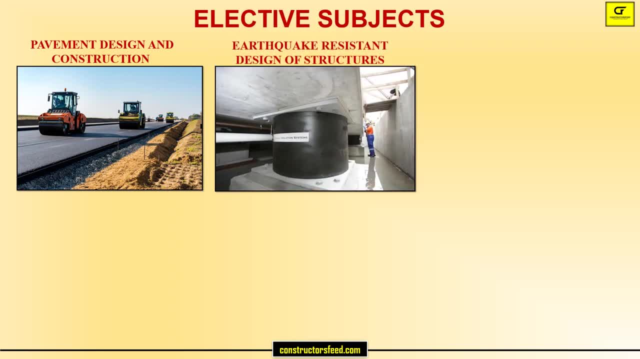 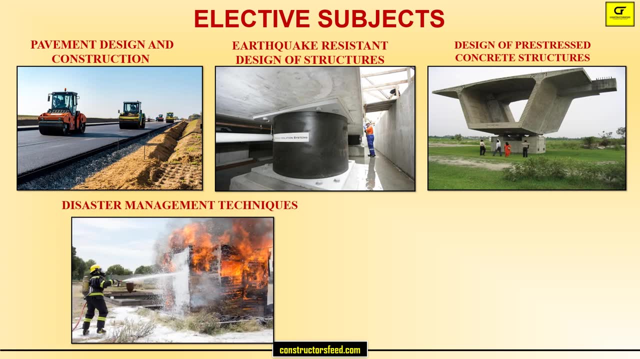 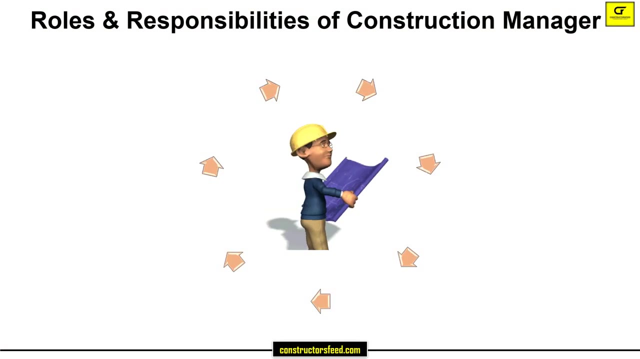 these are the reference books. elective subjects: pavement design and construction. earthquake resistant design of structures. design of pre-stressed concrete structures. disaster management techniques. advanced design of steel structures. some of the roles and responsibilities of construction manager: activity and resources planning, organizing and motivating a project team. controlling time management.